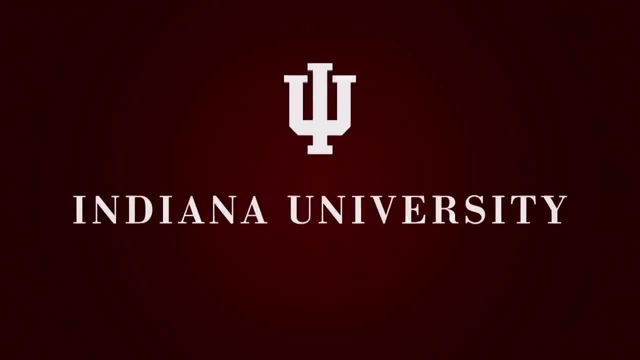 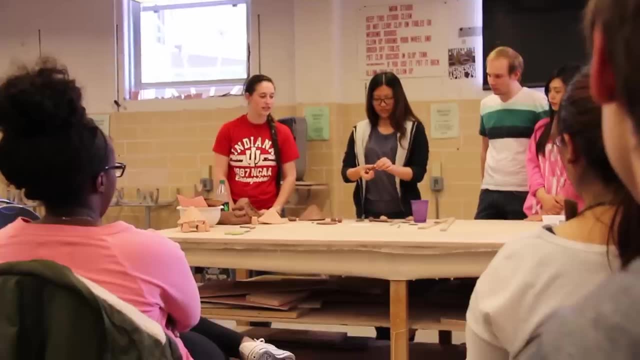 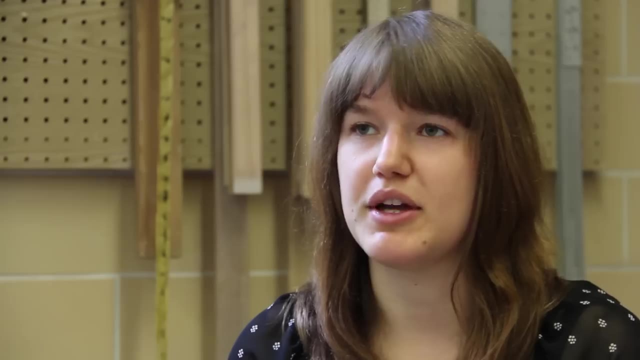 I think that students learn better when they actually have a chance to turn around and teach the material to someone else. So we came up with the plan that the Bloomington Clay Studio would host my students teaching a free class to patrons from Big Brothers, Big Sisters. 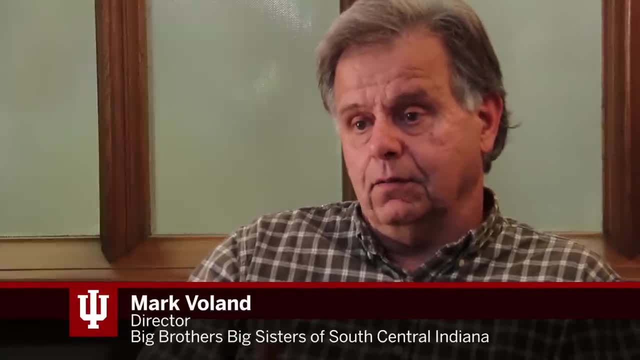 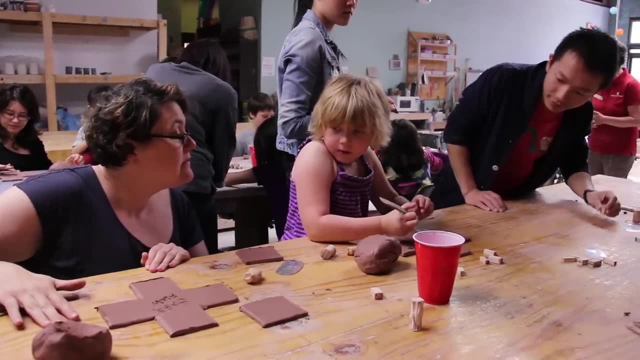 We felt that that was going to be a great opportunity for Big and Little to not only learn something new, but it also requires them to communicate with each other while they're working together. We're always coaching our Bigs to try to create new opportunities. 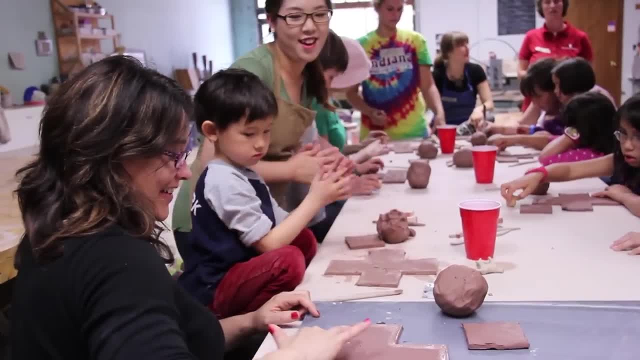 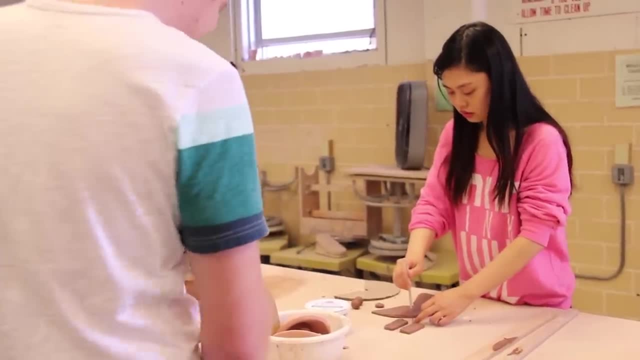 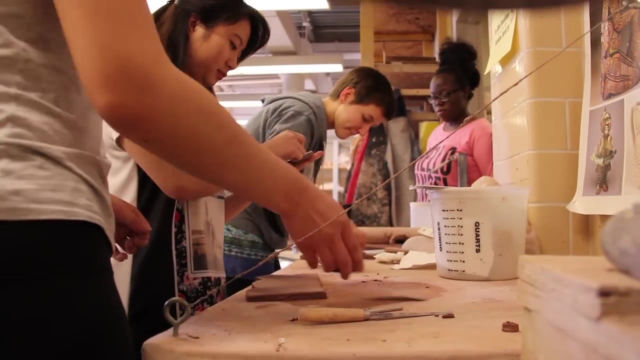 for their Little's and explore the community. This was our first opportunity in working with Clay, so that was really great. I wanted the students to go into these classes being really well prepared, So we actually started right around midterm with the project proposal and getting that together And then 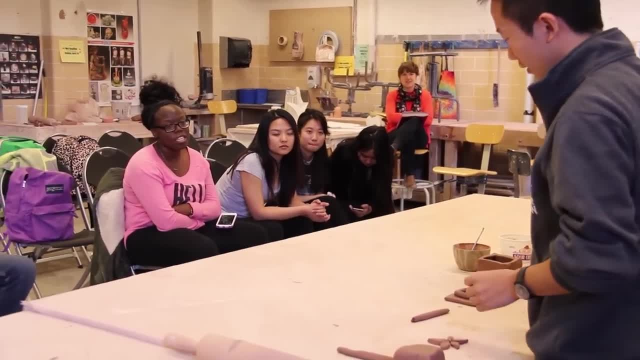 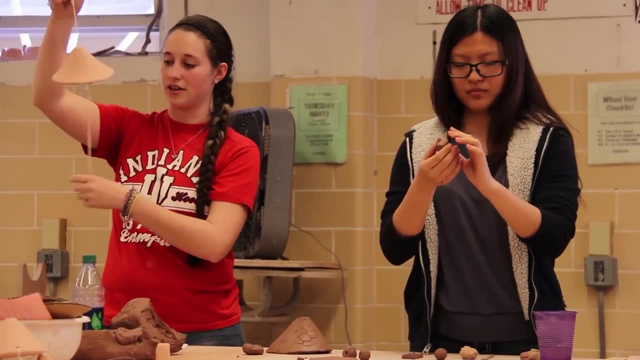 mid to late April we did the pretend And then the beginning of May was the actual class. There were three groups and each group came with a different project. So the first group- they made a wind chime- And the second: 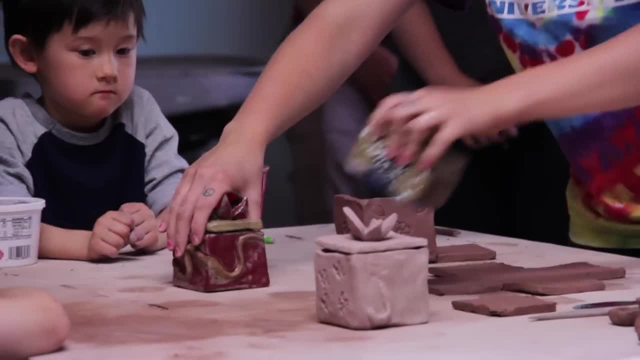 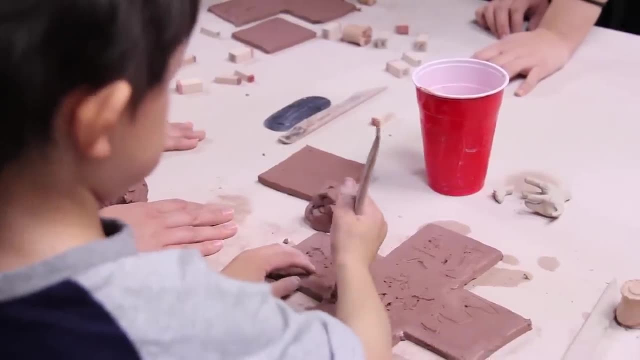 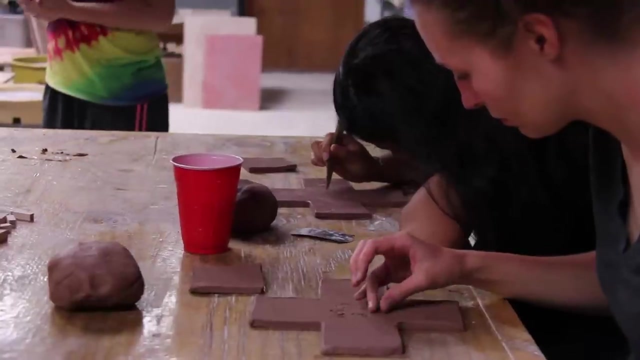 group they made a box which they called a magical mystery box. And then the final group, they made a little statue of a penguin. I think a lot of the kids really felt like they not only created something that was really neat and fun, but also that they learned a skill that they didn't know that they had. 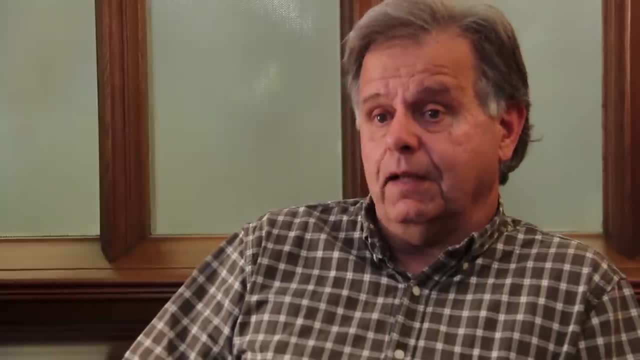 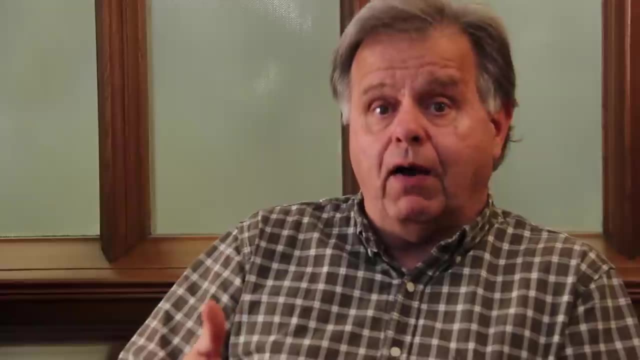 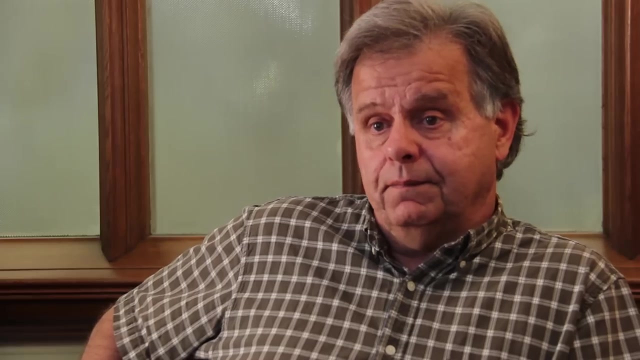 And I think we'll see that happen Down the line from here. a lot of these kids may pick that up as a specific interest in their life. So being able to interact with a college student they could say, wow, this is a class I could take at IU And that can really start a spark with them. 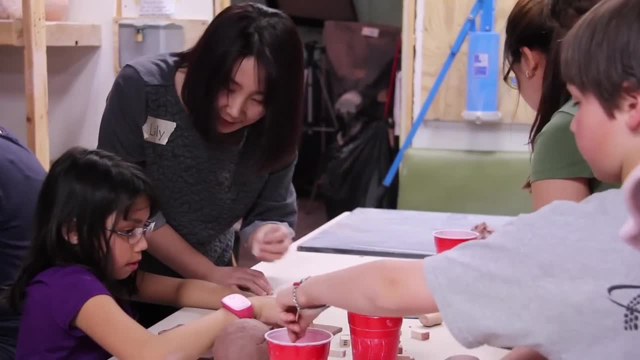 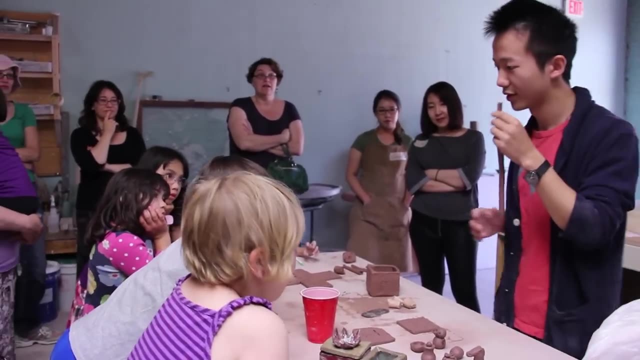 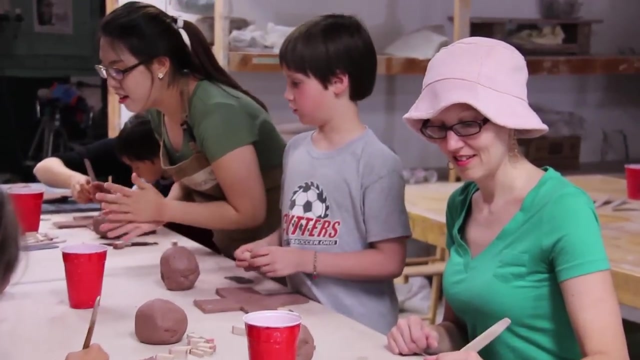 And I think my students learned a lot and the community benefited from this, And my main hope is that this isn't kind of the end of the project. I'm just thankful for everybody who put this together. Thank you. It's just a great thing, Anything that again the kids we serve, that the community comes. 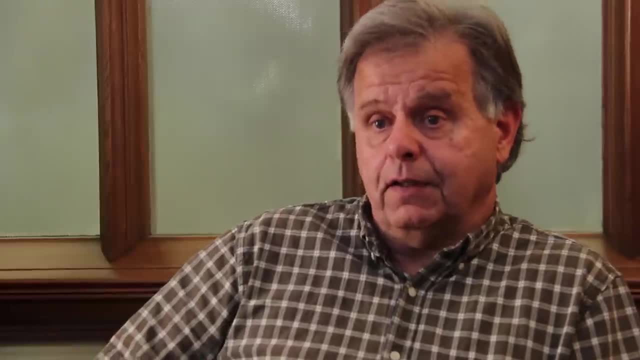 together to help. it makes this community better And that's really great for everybody.